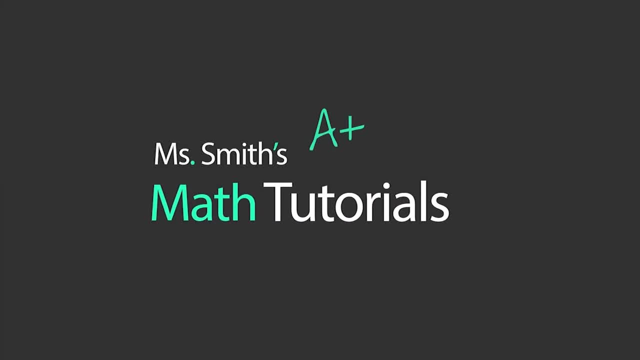 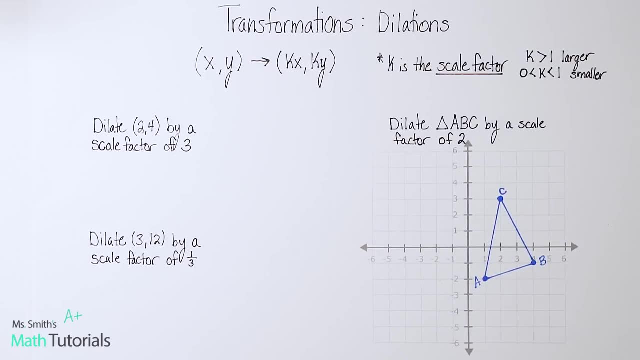 Welcome to Ms Smith's Math Tutorials. I'm Ms Smith. In this video we're going to be starting our transformations unit. This unit and these next few videos are going to be all about transformations. So the first transformation we're going to talk about is dilations. So 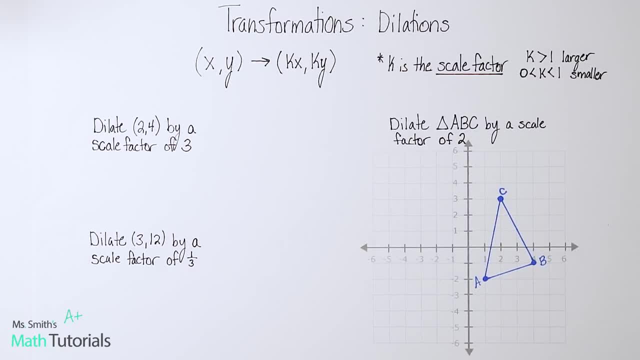 dilations are when we make something, a shape, on a graph, either larger or smaller. In this section of transformations, we're going to be giving you a lot of formulas, if you will, rules to follow for specific types of transformations. It's really beneficial to learn the rules. 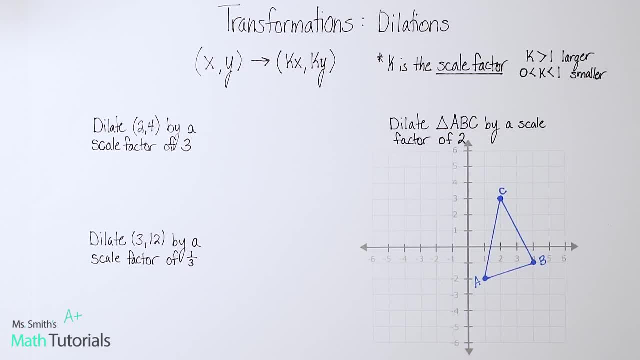 because you never know when you're going to have to go into a testing situation where you don't get a cheat sheet of the rules- and there are quite a few of them, So it is a good idea to try your best to memorize them. So the first one we're going to learn is: we're 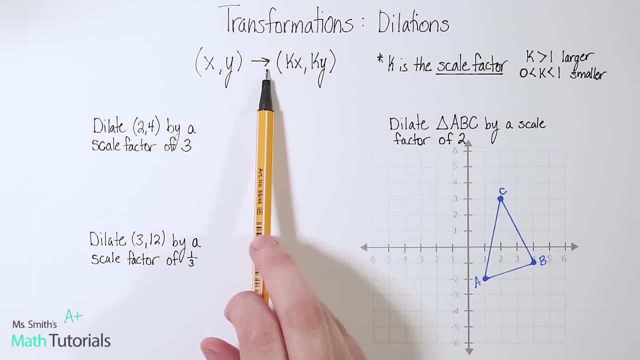 going to take a point, an x-axis. We're going to take any point and it will become that's kind of how this reads. xy becomes in this case, for dilation, the rule is k times x and k times y. Now k is the scale. 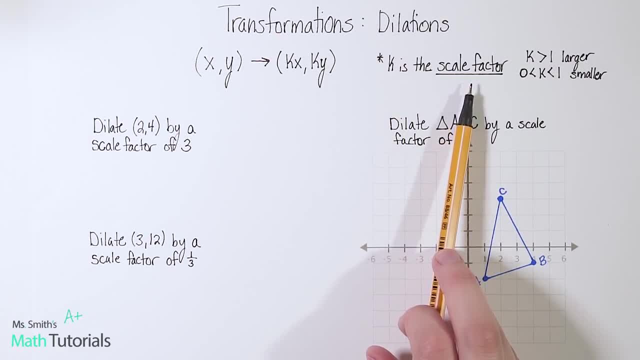 factor. Okay, so k is how big or how small we're going to make something. So here are the rules. If k is larger than one, if k is greater than one- so anything bigger than one- 1.5,, 2,, 3, anything greater- then our shape is going to get larger in size. It's. 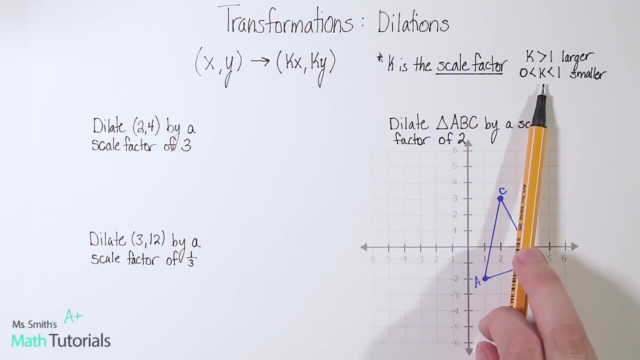 going to get bigger, Okay, but if k falls between 0 and 1, meaning it's a fraction or decimal less than 1, for example, 1 half, 1, third, 3, fourths, okay, 0.75, if it falls. 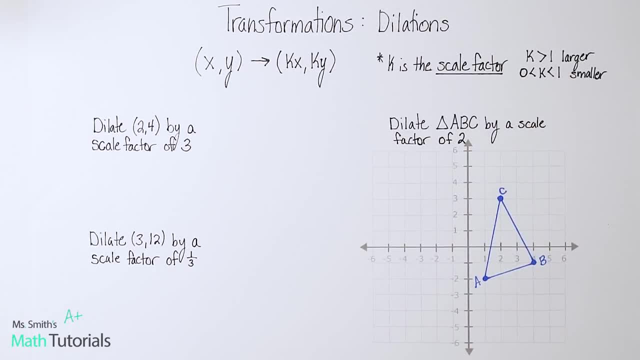 between 0 and 1, that means our k is larger than 1.5.. Our shape or picture is going to get smaller, So you'll be able to, once you get the hang of it, really quickly identify, just by looking at it, if something's going to get larger or 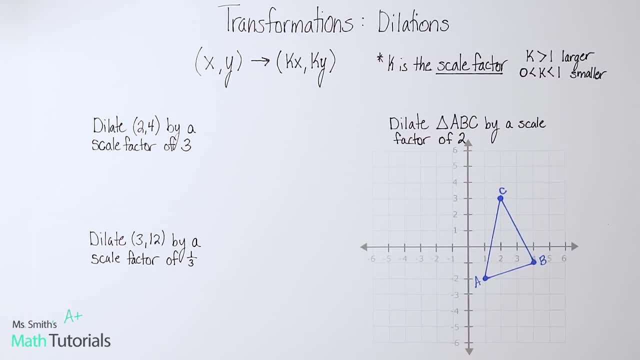 smaller, based on the scale factor. So, coming back to the rule, so we're going to take that scale factor, which they'll give us in whatever problem they're asking you, and you're just going to multiply it by your x value and multiply it by your y value. All right, so let's see. 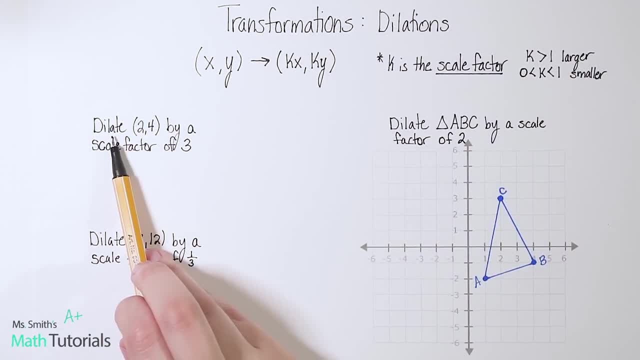 this in action. We're going to start over here. Our instructions say: dilate this point 2, 4, that's an x- y point- by a scale factor of 3.. Okay so, if 3 is my k in this instance, so I'm going to. 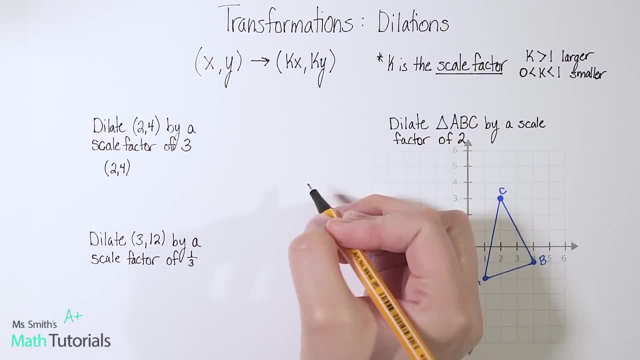 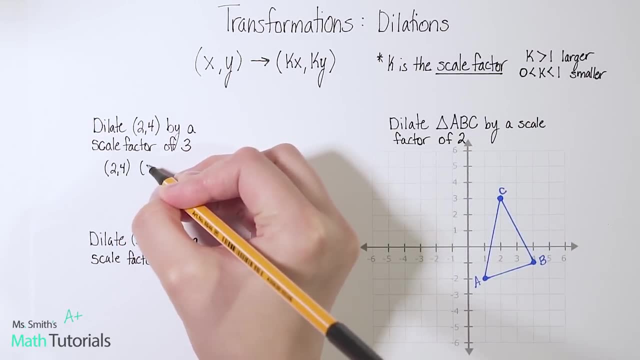 take the point 2,, 4,, all right, and I'm going to multiply each of these by 3.. So that'll be 2 times 3, comma 4.. Times 3.. All right, and let's write our final answer. So 2 times 3, we know is 6, and 4 times. 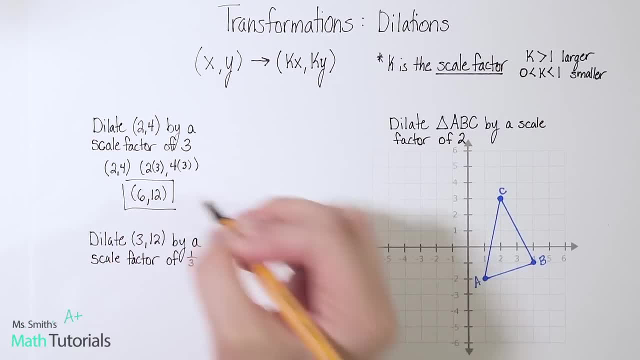 3 is 12.. So notice that our numbers did get larger because our scale factor was greater than 1.. 3 is greater than 1, so we went larger. Okay, now let's try this one. Dilate 3, comma. 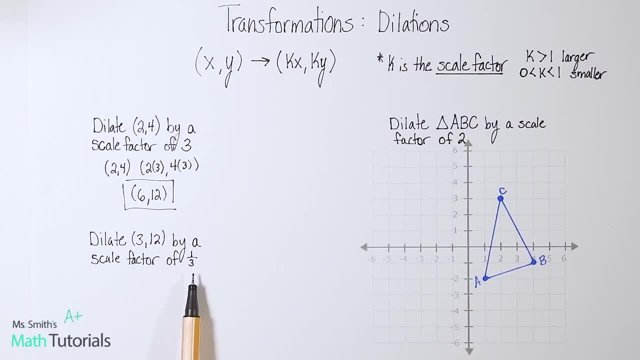 12 by a scale factor. Okay, so we're going to take that original point 3,, comma 12.. We're going to take the 3 and multiply it by 1 third, and we're going to take the 12 and multiply it by 1 third. 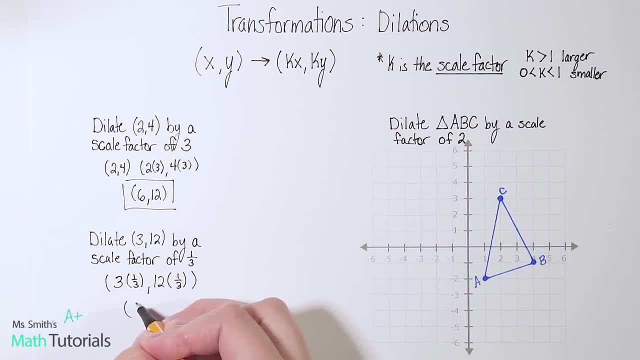 Okay, now, 3 times 1 third is just 1.. Okay, 12 times 1 third is going to give us 4.. All right, so notice how our point became smaller, because our scale factor was between 0 and 1.. Okay, it was 1 third. 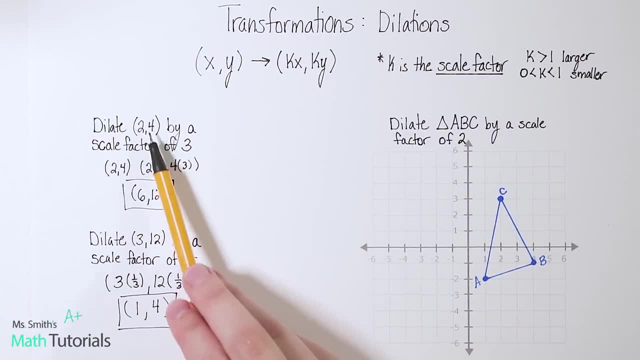 Now let's see how this would look with an actual shape. So we've gone point by point. but now let's look at if I had a sequence of points, if I had an actual picture to work with. So my instructions say: dilate 3 by a scale factor. So I'm going to take the 3 and multiply. 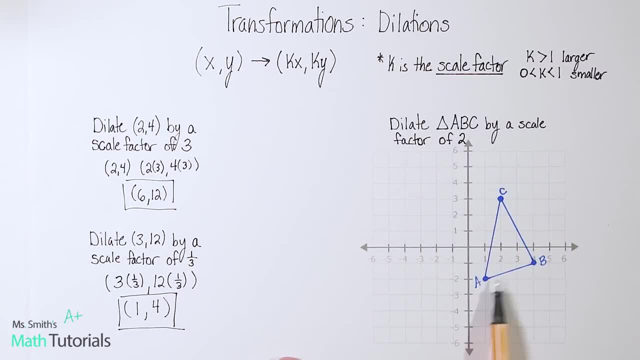 it by 1 third. Okay, so I'm going to take the triangle ABC. So here's triangle ABC by a scale factor of 2.. So hopefully you're noticing that 2 is larger than 1, which means my side, my 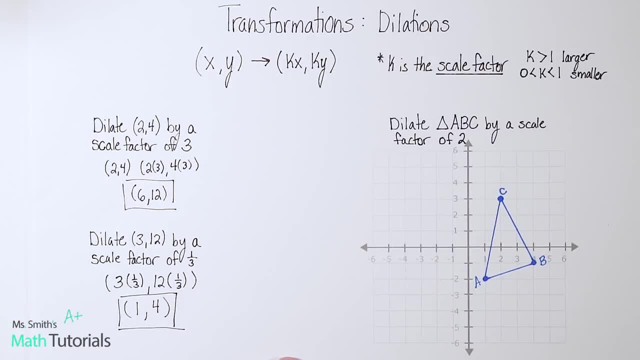 my triangle should get larger than it currently is, but we'll see. So I first need to figure out what are the points I'm working with, right, I need to lay out that information first. So we'll start with A. Point A is Falls at 1 negative 2.. So let me know if that worked. And 3 is separate Products are just분 larepod and machine attempting. They're pretty close apart. Now, if someone has converted in the other ear, know the rules and fallen yet again, Take a 1991 dot and write was plus 0. You substitute Lyndりました studenthvi klaaceacsa. 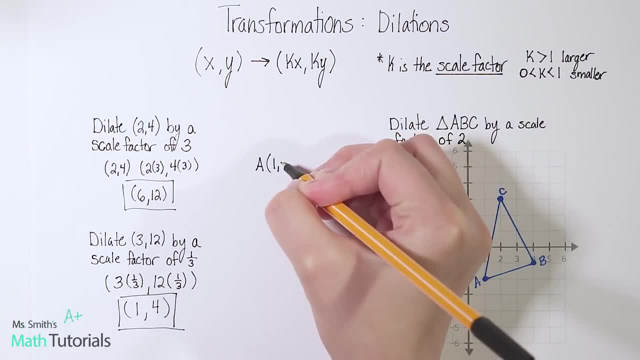 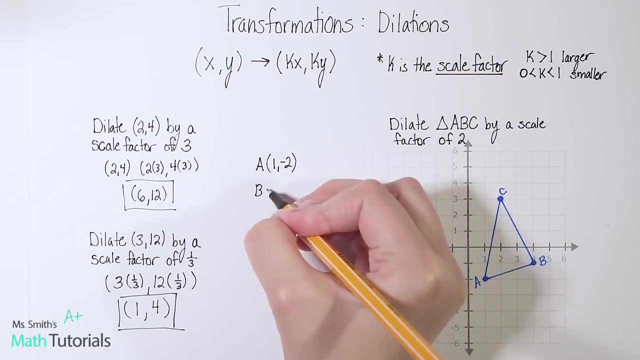 here: A falls at 1, negative, 2.. B falls at 4, negative. 1.. C falls at 2, 3.. Okay, so that's where my points currently are. so I'm gonna follow this rule, remembering that my scale factor is 2.. So I'm gonna multiply each X and each Y by 2 to get a. 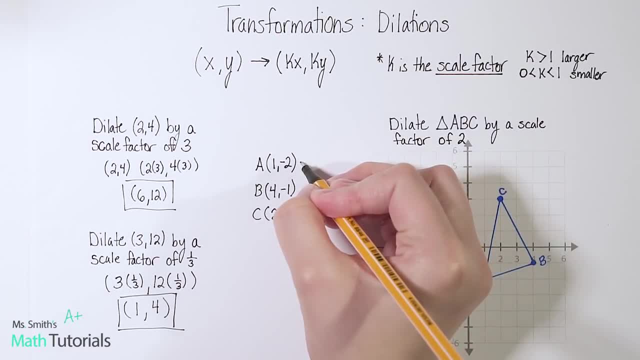 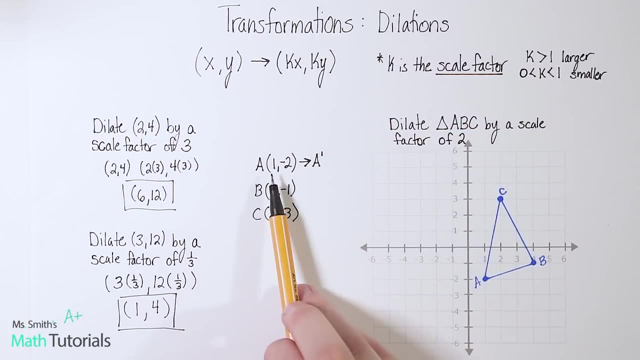 new point. So this A is going to become now the way we write this in math is we say A prime. So let's follow that rule: 1 times 2 is 2 and negative 2 times 2, that would give me negative 4.. So that's gonna be my. 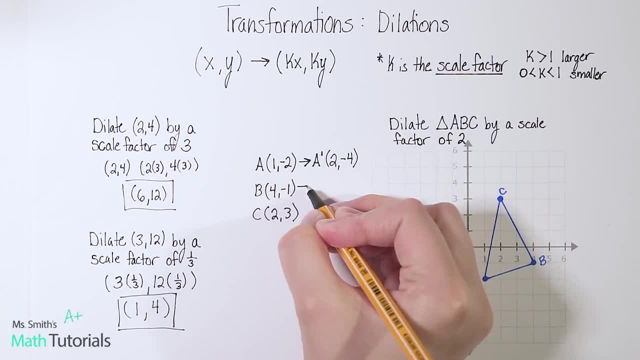 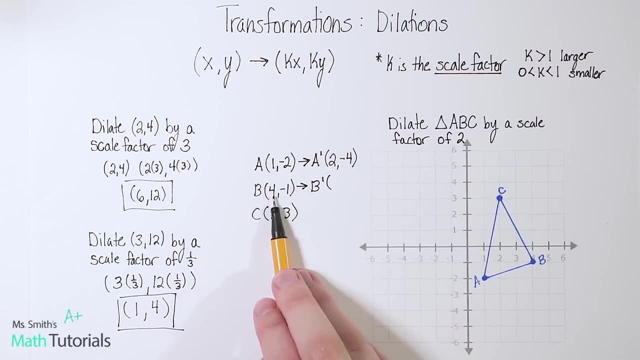 new point for A, So let's do the same thing with B. So we'll call this B prime. So 4 times 2 is going to be 8, and negative 1 times 2 is going to be negative 2.. Alright, and now we'll do our new C. C prime is going to be 2 times 2. 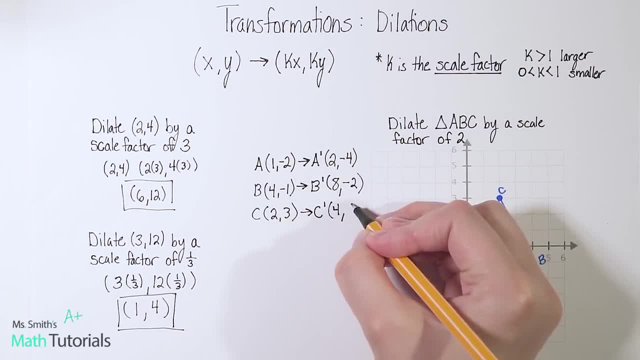 is 4 and 3 times 2 is 6.. Okay, now let me graph my new image. You'll notice- you may have realized it, and I just realized it- that I've got an 8 here, but my graph only goes up to 6.. That's okay, we're just gonna estimate. I just made a careless 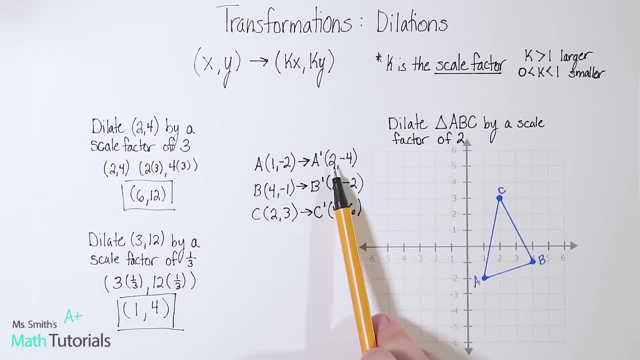 error when I was making this. So let's do A: prime would be at 2, negative 4.. So 2 down 4.. And we'll label that A prime. Okay, B, and I should note that labeling is so important. Okay, if you've just plotted a point.